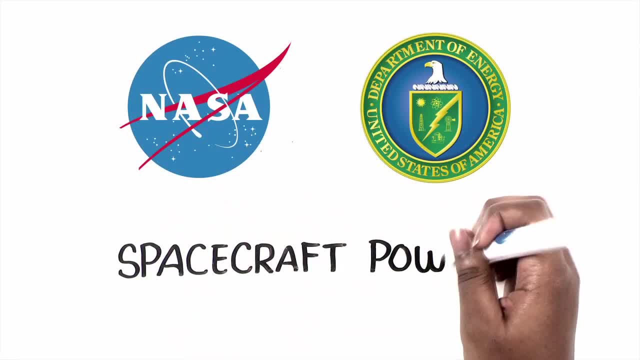 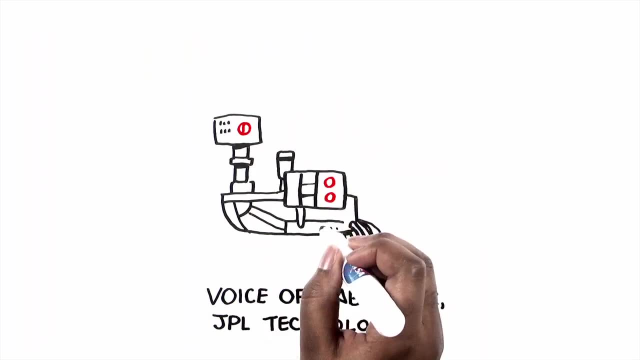 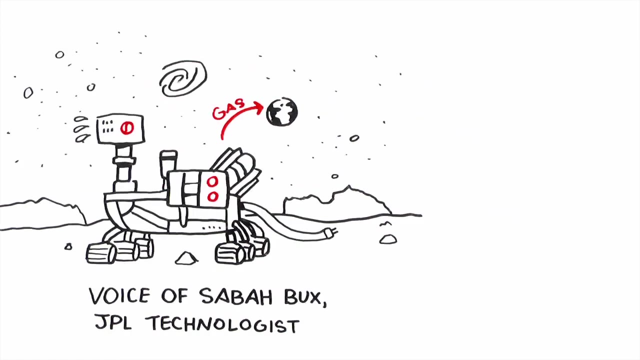 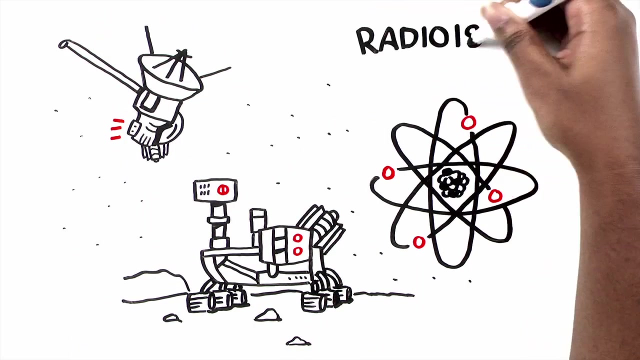 If you want to drive a rover on Mars, you have to keep in mind there's no gas station for millions of miles and there's no outlet to plug into for power. That's why NASA's Curiosity rover on Mars and other NASA spacecraft that explore the solar system use something called radioisotope power. 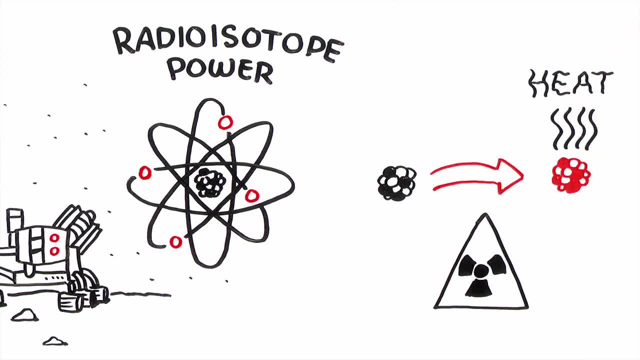 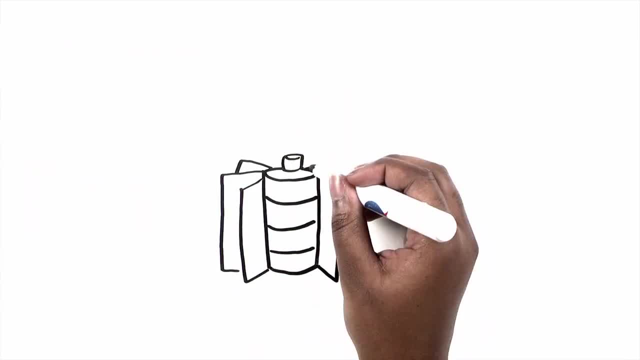 A radioactive substance releases heat as it breaks down or decays. A system that converts that heat into electricity is called a radioisotope power system. These systems get fancy names. Curiosity's power system is called the MMRTG multi-mission radioisotope thermoelectric generator. 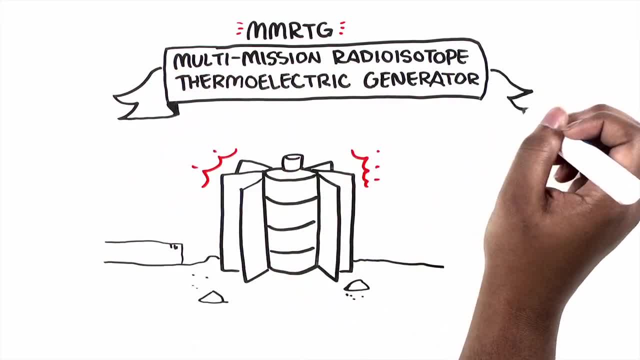 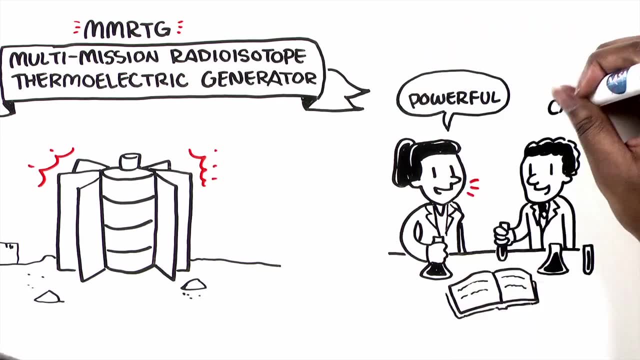 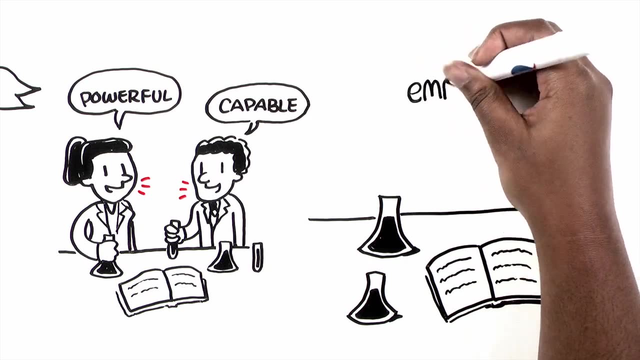 MMRTGs are reliable and last a long time. NASA's Jet Propulsion Laboratory is working with the Department of Energy on ways to make them even more powerful and capable. So researchers want to make the next generation of radioisotope power systems the EMMRTG. 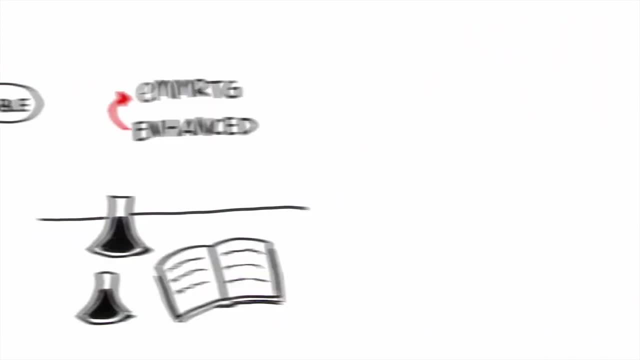 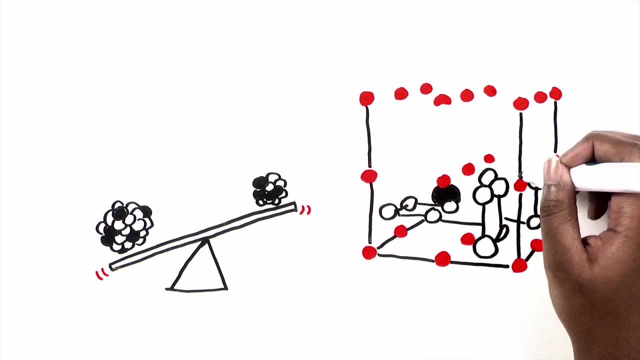 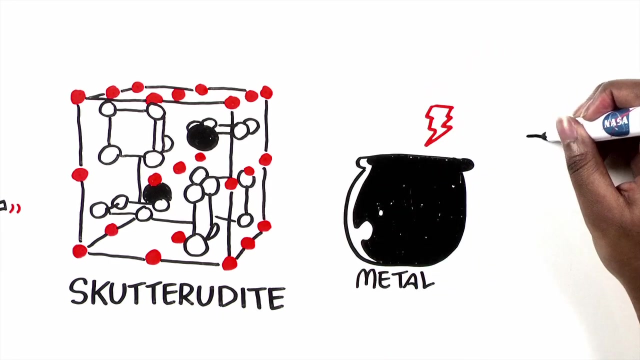 The E stands for enhanced. The new thermoelectric technology in development is based upon materials called scuttererudites. They are a part of a family of compounds with many heavy atoms and complex structures. Scuttererudites conduct electricity like a metal, but insulate against heat the way glass does. 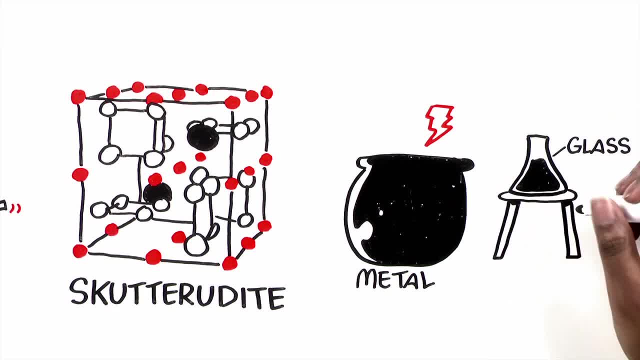 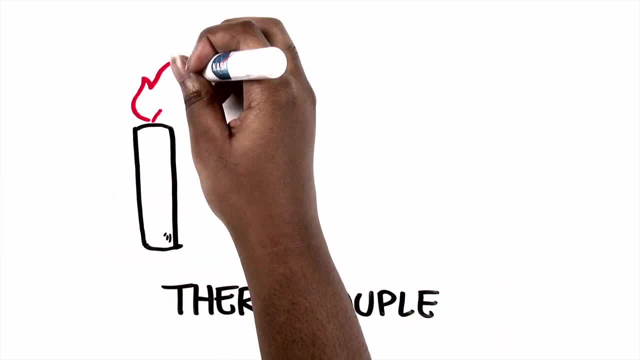 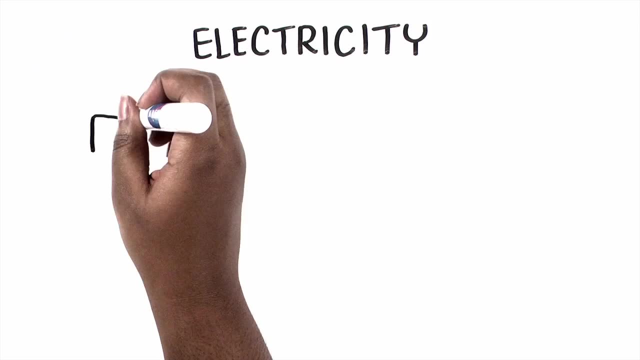 At the same time, they can generate sizable electrical voltages, just what engineers need to convert heat into electricity. Engineers use this material in devices called thermocouples, which are used to generate electricity. One of the thermocouple's shoes is hot and one is cold. 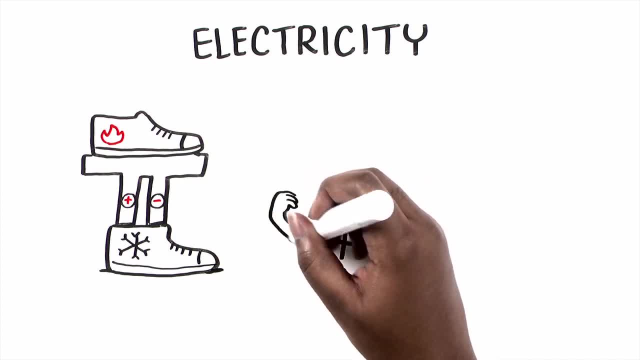 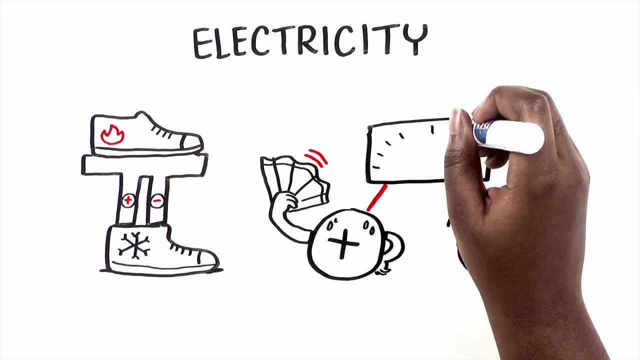 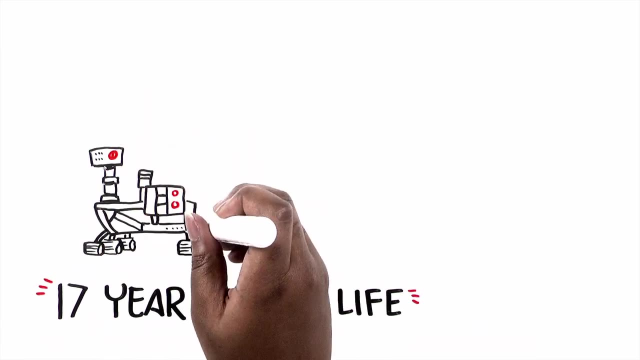 This heat, transferred across a big temperature difference, makes electrical charges flow from the hot shoe to the cold shoe and produces an electrical voltage And this generates useful electrical power. If these materials were put in the same kind of generator- that's on the Curiosity rover with some small tweaks- 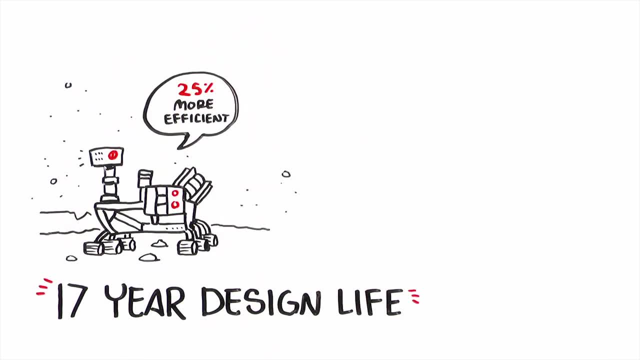 the generator could be up to 25% more efficient. After 17 years, a spacecraft could have 50% more power than with the current design. That means a spacecraft with an EMMRTG could fly longer and do more science during its lifetime.